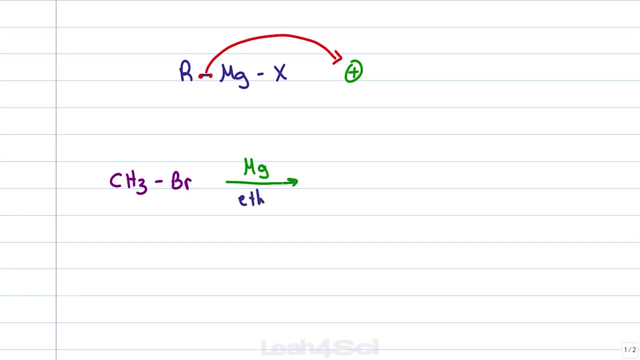 this alkyl halide and react it with magnesium, typically with something like ether. The solvent you use is very important because you are not allowed to use a polar product solvent. More on this in a minute. The Grignard that forms has our initial carbon chain, the methyl group. 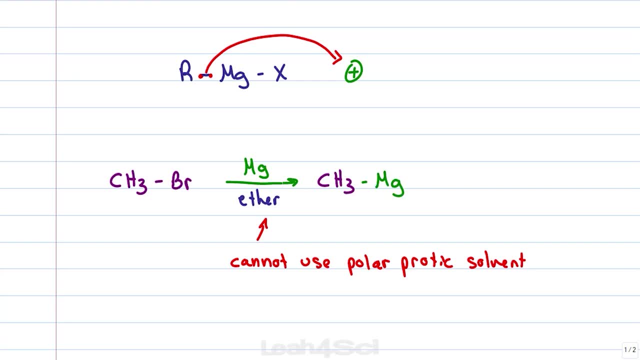 with the magnesium inserted between the carbon and halogen. This right here is a methyl Grignard, with the methyl carbon being the carbanion like ready to attack group. I show this with a bromine, which is most common, but you're also going to see it with iodine and chlorine, Where bromine and 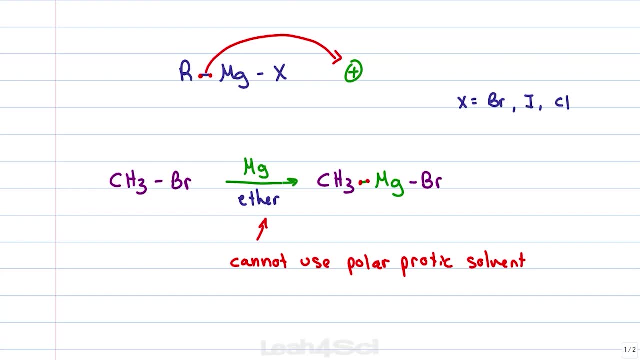 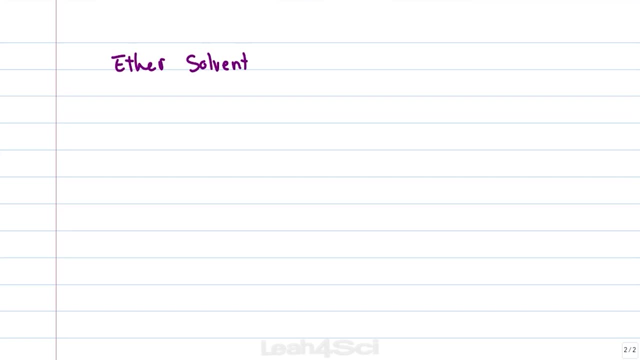 iodine react quickly and chlorine a little bit bit slower. So why do we use an ether solvent? First, make sure you review my polar, protic and aprotic solvent video link below and then take a look at ether compared to something like alcohol. 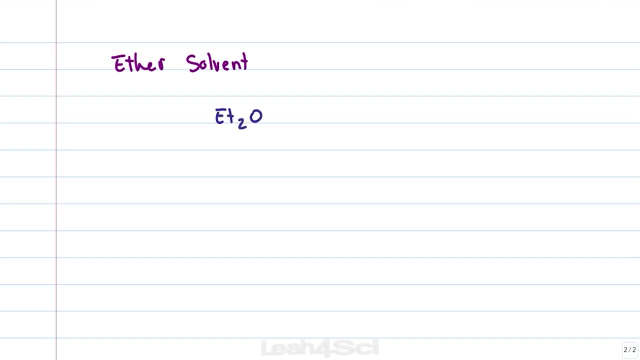 The common ethers you'll see for Grignard formation are ET2O, which is diethyl ether, or THF tetrahydrofuran, which is a heterocyclic ring with an oxygen in it. Compare this to other common solvents that you're used to seeing, like water or alcohol. Remember, the Grignard is so reactive. 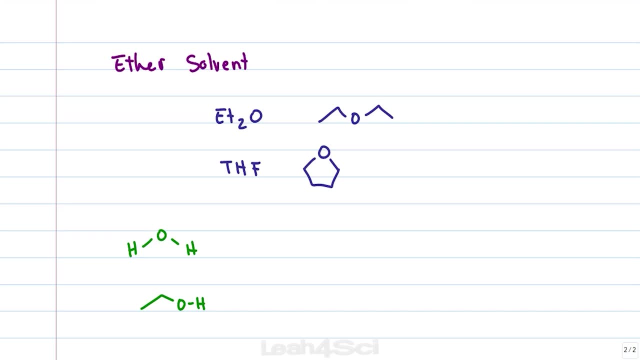 it wants to attack anything and everything. So let's say I have a reaction and I manage to form a Grignard with a CH3 bound to the MgBr and it's dissolved in water. The problem is water has a partially negative oxygen atom and partially positive hydrogen. so if that Grignard somehow manages to form that oxygen atom, it will eventually get dissolved in water. So if it'sung in water, it'll melt down in water and the reaction is negative because it will have a wholly positive hydrogen. and if it has a partially negative hydrogen atom, it will have a positively positive. 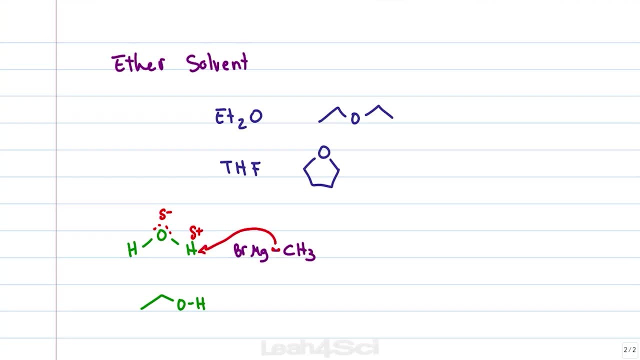 Then now the new Grignard reagent immediately takes advantage of its carbanion-like state, attacks the hydrogen atom from the protic solvent, giving oxygen back its electrons and giving me something that looks like this: Our purple CH3 from the Grignard is now bound to the green hydrogen from water in solution. 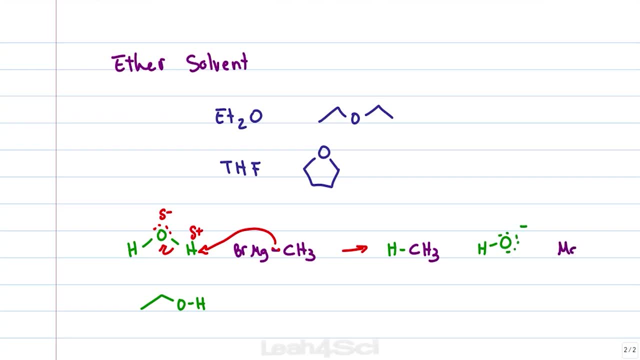 we also have an OH- and the useless MgBr plus just floating around the solution. So sure, we created the Grignard, but we immediately destroyed it and got nothing out of it. Think of this almost like sending a little kid to the ice cream store: go get me an ice. 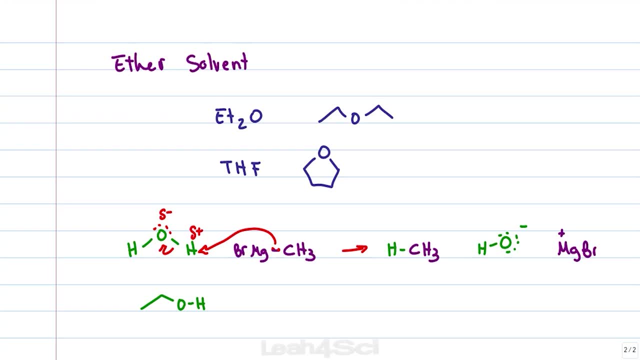 cream. The kid's gonna go. he's very happy. he gets the ice cream, but he eats it on the way. Did he do what you asked? Yes, he got the ice cream. Did you get anything? No, because he ate it. 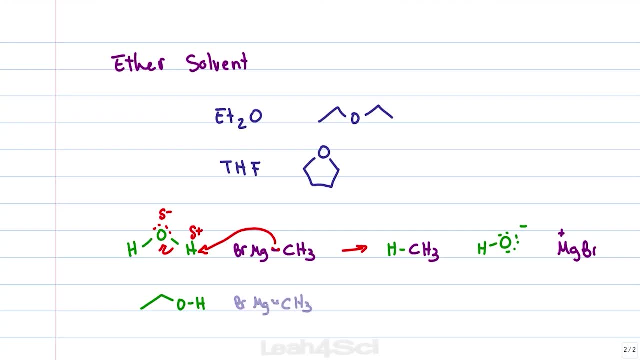 Your ice cream is gone. Same thing for something like alcohol. the Grignard will attack the hydrogen, give oxygen back its electrons. Once again, I have CH3 bound to an OH-. I have an OH- in solution. Grignard is destroyed and I'm left with N-alcoxide and an MgBr plus. 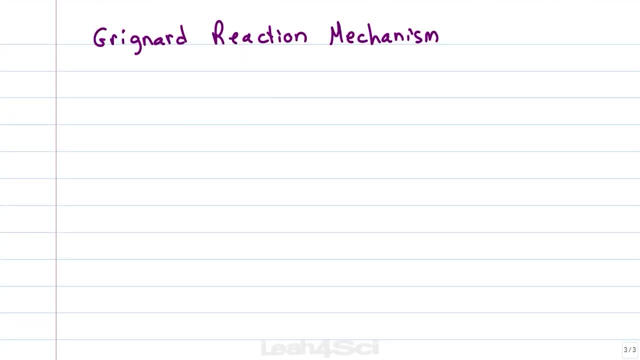 Now that we know what not to do, let's take a look at the Grignard reaction mechanism, starting with an Ethyl Grignard reacting with acetone. Since Grignards can attack many compounds, I created a mini cheat sheet that you can. 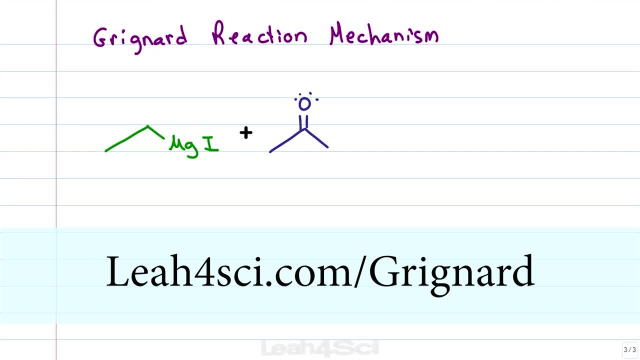 find on my website, leah4scicom: slash Grignard. The most common is the carbonyl. that gives you an alcohol And the mechanism looks like this. Carbonism looks something like this: First, remember, the bond between carbon and magnesium is the bond that's going to attack. 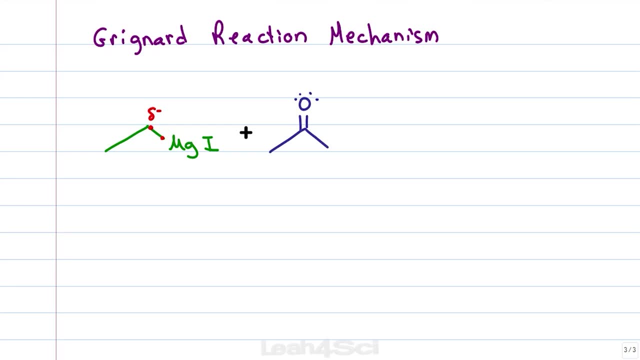 because this is the carbon that's very carbanion-like. Recall that in a carbonyl we have resonance between the carbon and the oxygen, making the oxygen very partially negative and the carbonyl carbon very partially positive. The Grignard reaction begins when the carbanion-like electrons are going to reach out and attack. 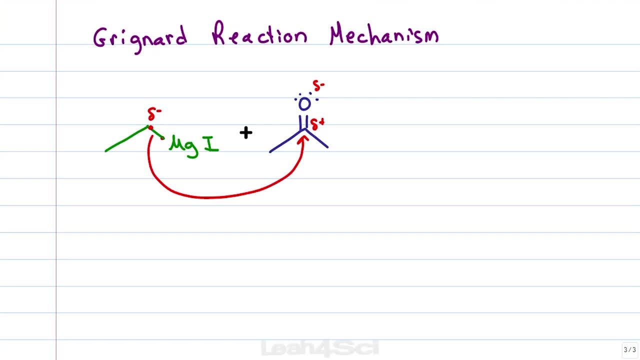 the partially positive carbonyl carbon. This would put a fifth bond onto carbon, which can't happen, and so the pi bond is going to get kicked up onto the oxygen atom. What we get is a carbon chain as before, with only one bond to oxygen. 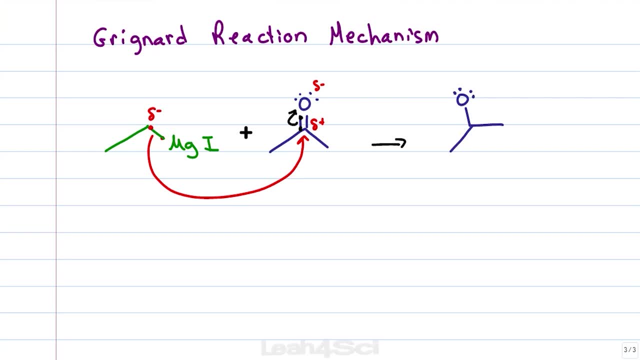 Oxygen had two pairs of blue electrons and now gets a third pair of black electrons with a formal charge of minus one Attached to the carbonyl carbon. We now have a new bond To the ethyl group, which is from the ethyl Grignard. 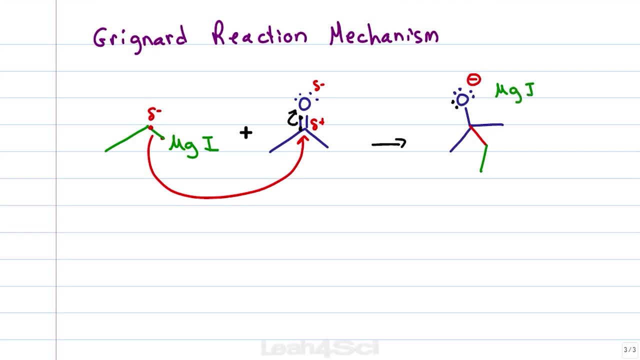 Off in solution. we also have the MgI plus and many professors like to see it drawn next to the oxygen to show the counter ion pair. But we're not done because oxygen still has a negative charge. so let's add in acid which you can just write as H3O plus, and I'll draw one of the H pluses here. 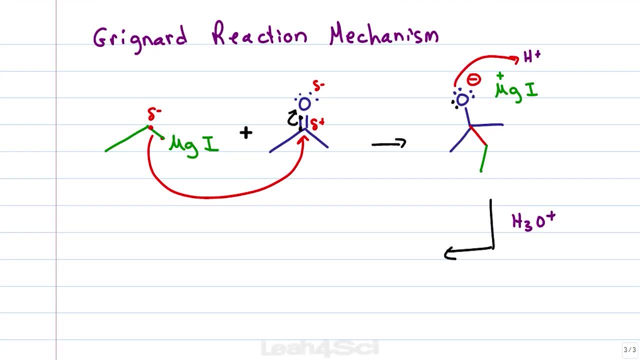 The negative oxygen reaches for the hydrogen To give me an alcohol as the final product. This looks a little messy, so if you want to redraw it, our longest carbon chain has four carbons: One, two, three, four, with an alcohol on carbon two and a methyl group also on carbon two. 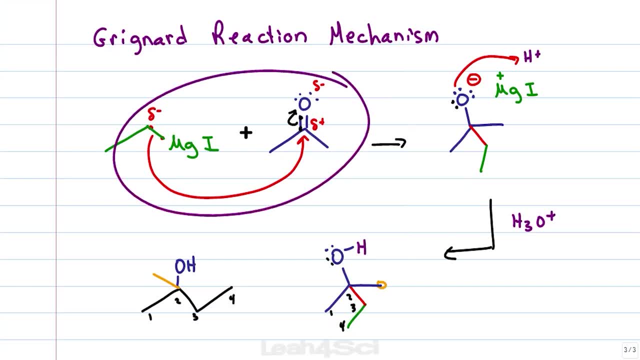 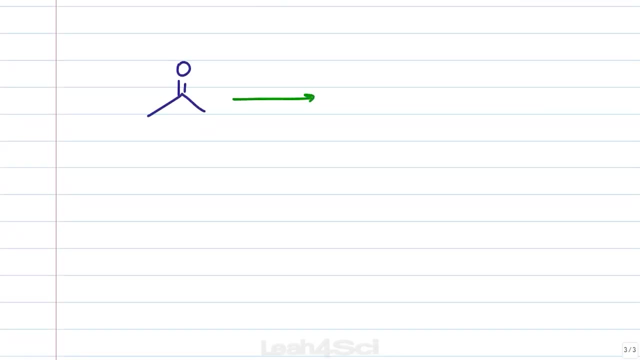 Notice that, as we did this mechanism, we had the Grignard attack happen first and only when it was done, when we already had the irreversible carbon to carbon bond formation is when we added the water. If I were to write out this reaction with the steps instead of the mechanisms, and I 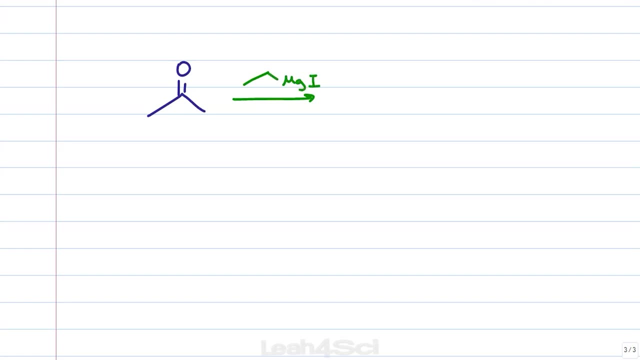 drew it like this, with an MgI and then added H3O plus. this would be completely incorrect. Remember: Grignards are going to attack acidic or polar product groups and that will destroy your Grignard. To make sure you get full credit, add the one to show that the Grignard attack is the 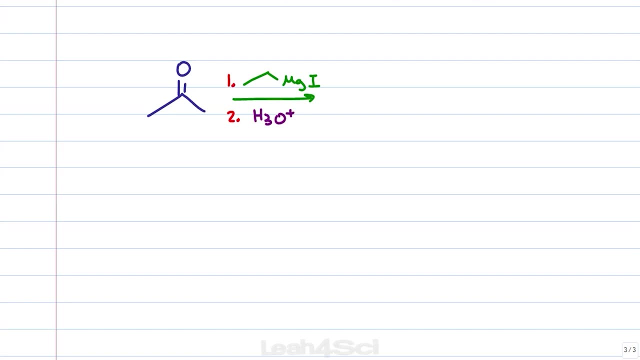 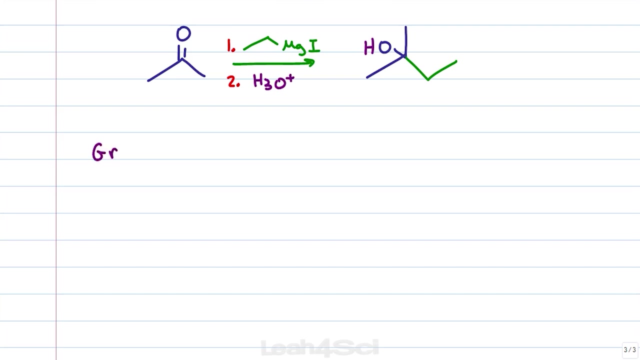 first step, And then two, Two, Two you a final step after the reaction is done, to give the final alcohol product. Now that you've seen the mechanism and overview of the reaction, here's a shortcut for both coming up with a Grignard product and recognizing what happened if you're given the product. 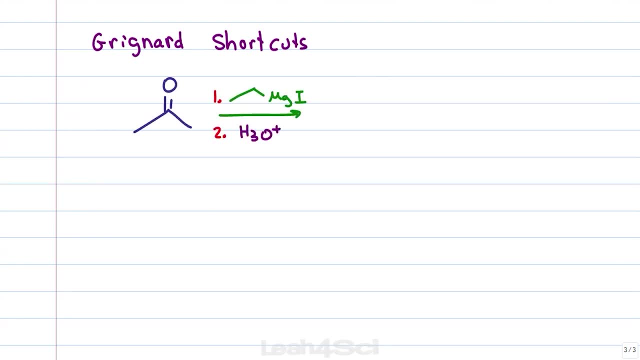 and have to come up with the reactants. If you see this question on the exam, very simple: identify your carbonyl carbon, break the pi bond and, on the carbonyl carbon, add the Grignard carbons one, two. 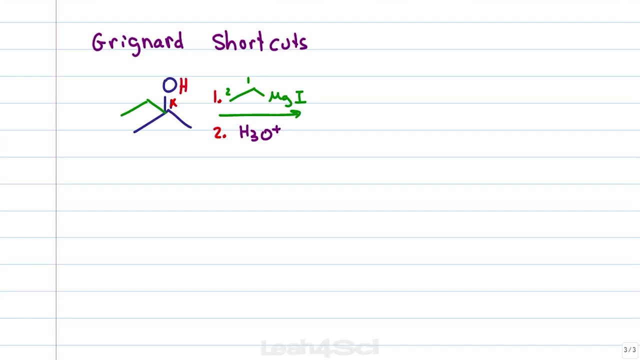 Then make sure you add a hydrogen onto the oxygen to form your alcohol. and there we have it. It's a little bit messy, but if you count one, two, three, four, a methyl group and an alcohol on carbon two, One, two, three, four alcohol and methyl on carbon two.